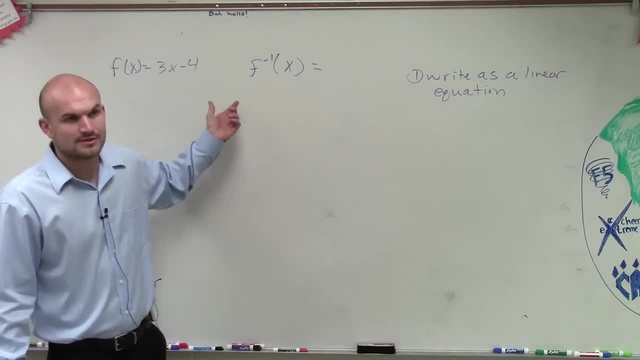 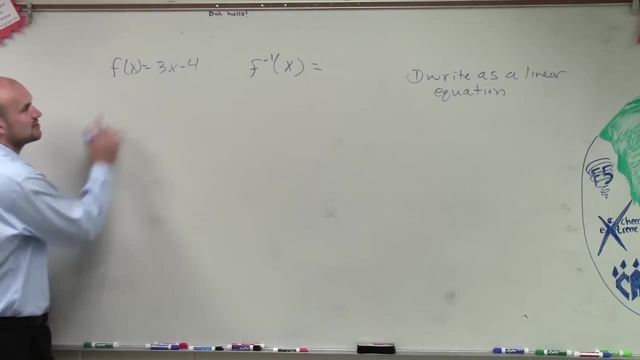 equation. You didn't have it as a function, You just already had it as a linear equation. So to find the inverse, you already would have to write it in a linear equation. So the first thing we want to do, if I'm given f of x equals 3x minus 4, to write it as a linear equation. I'm just going. 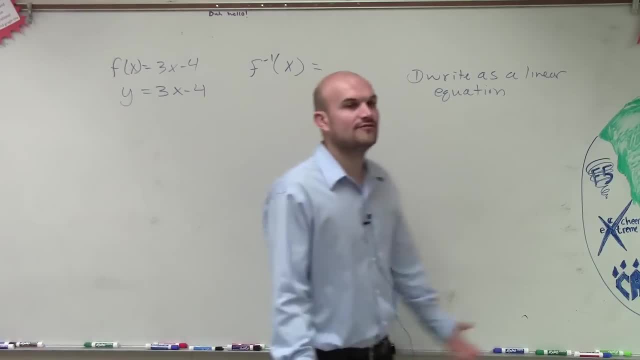 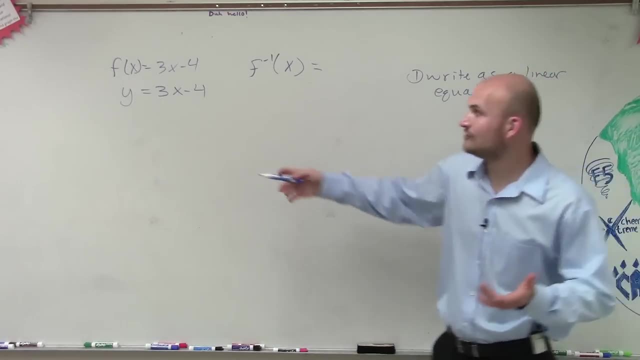 to use x and y's All right. so the first step is just to write it as a linear equation, Because we don't want to do mathematical operations with f of x, even though f of x and y are both your output values if you were to graph it. But we want to deal with y Because step number 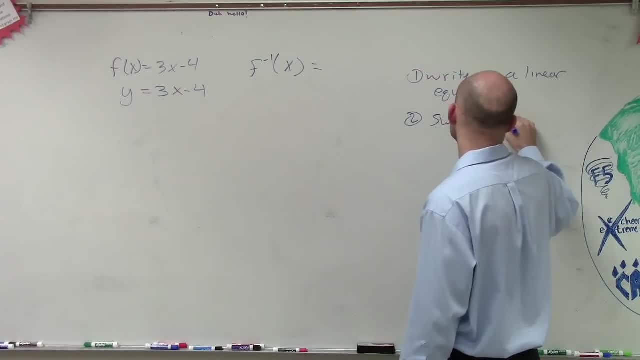 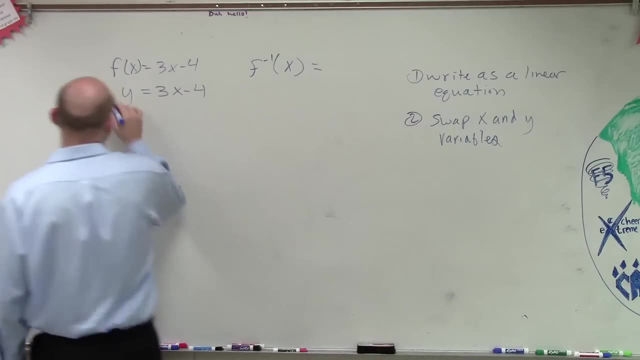 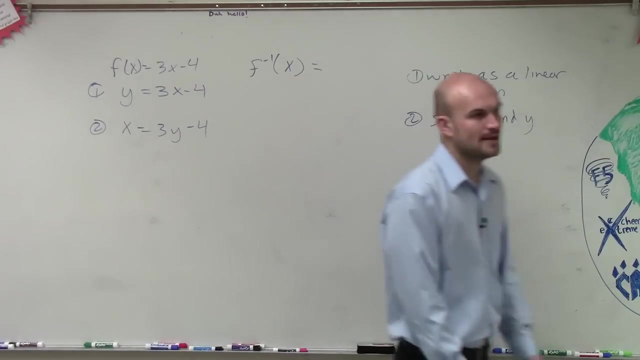 two says to swap your x and y variables. So now we'll swap x and y. So this was step one. Step two: you just swap x and y. Step three: solve for y. So now what we do: solve for y. So you add four to both sides And 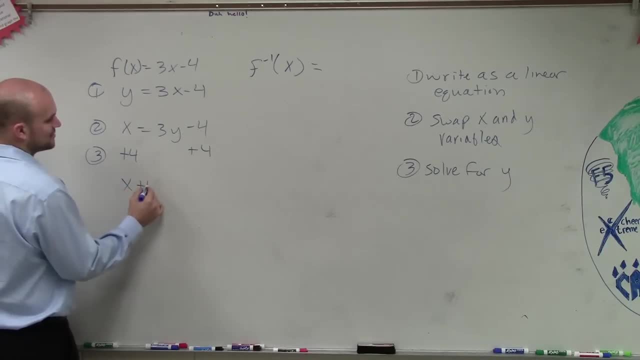 remember, this is a literal equation, So you're not going to be able to get a value. So it'd be: x plus 4 equals 3y, Then divide by 3.. So therefore not yet. So therefore we have x plus 4. 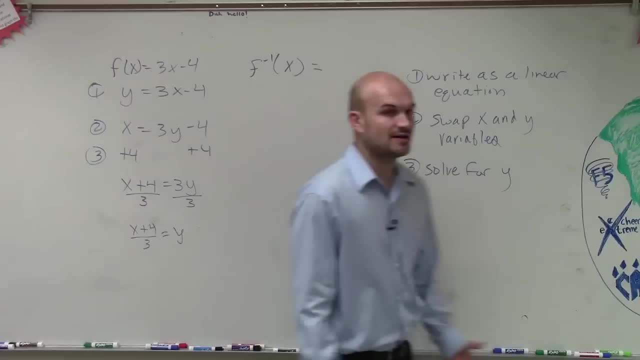 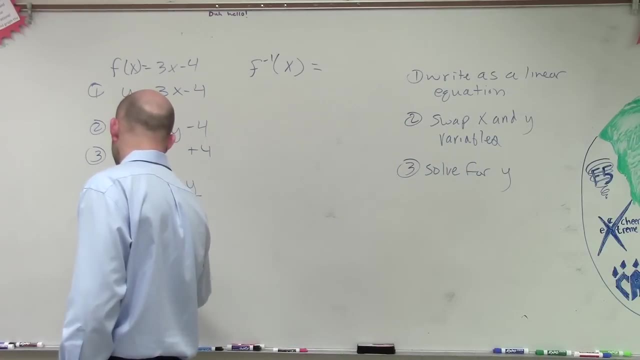 divided by 3 equals y. So I've done now step number three. Can't you simplify that though? We can rewrite this? We can write the y first and write it as 1 third x plus 4 thirds If. 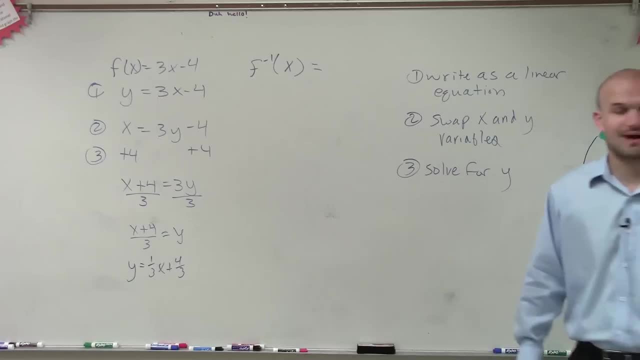 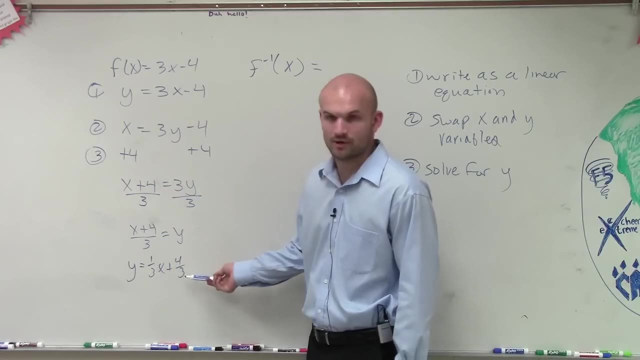 we were going to graph it, if you guys remember graphing it, remember I asked you to graph the inverse. This might be a little difficult to graph, So one thing we can do is divide the 3 into both of those terms. So then we have a slope and a y-intercept, But for this 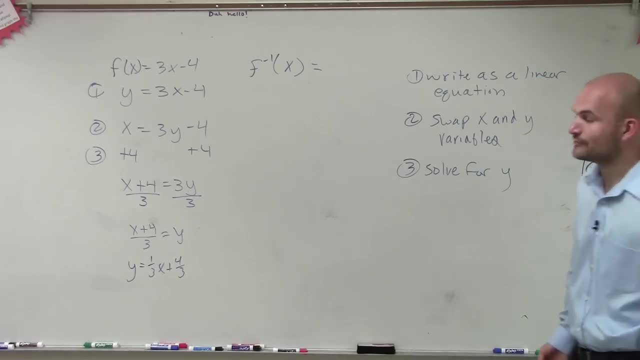 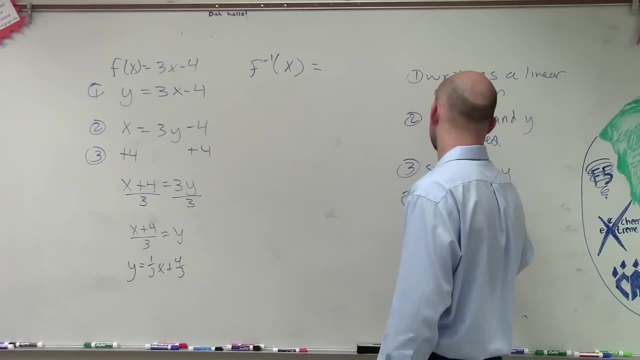 case, I'm not asking you to graph it, So leaving it in that form is fine, But if you were to graph it, you might want to remember how to do that. And then the last step 4, write in inverse notation. So inverse notation, ladies, and. 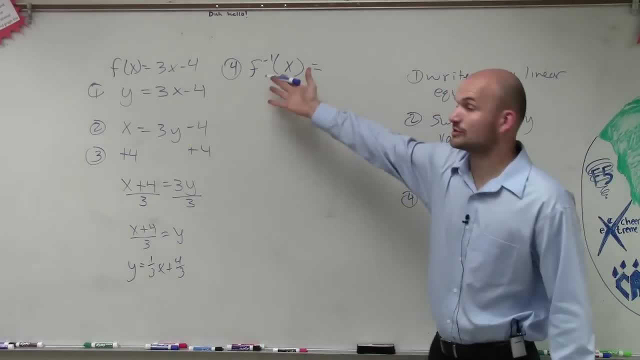 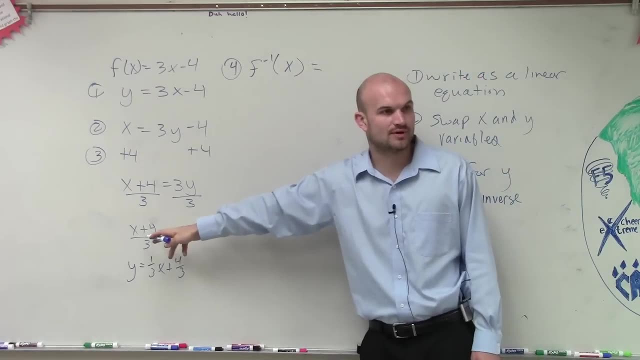 gentlemen. So originally, if I had a function f of x equals 3x minus 4, inverse notation looks like this: f inverse, with that little negative 1 of x equals. what did we say? What did y equal x plus 4.. 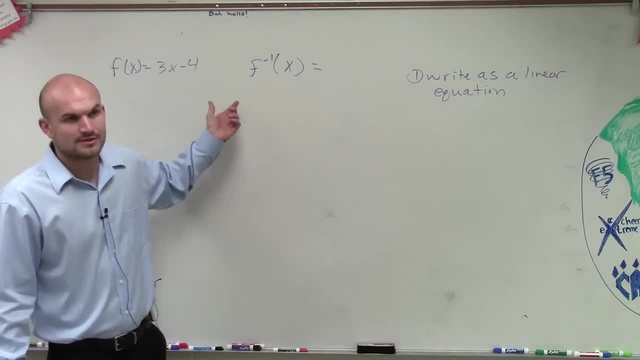 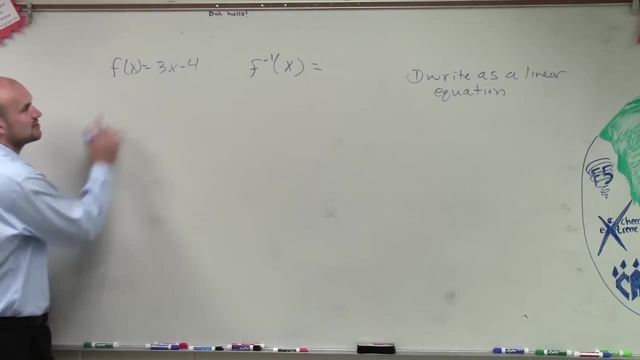 equation. You didn't have it as a function, You just already had it as a linear equation. So to find the inverse, you already would have to write it in a linear equation. So the first thing we want to do, if I'm given f of x equals 3x minus 4, to write it as a linear equation. I'm just going. 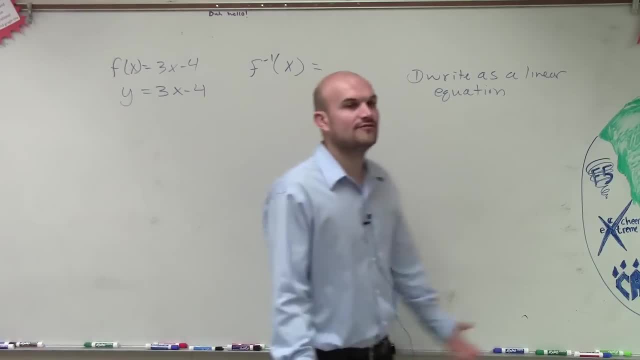 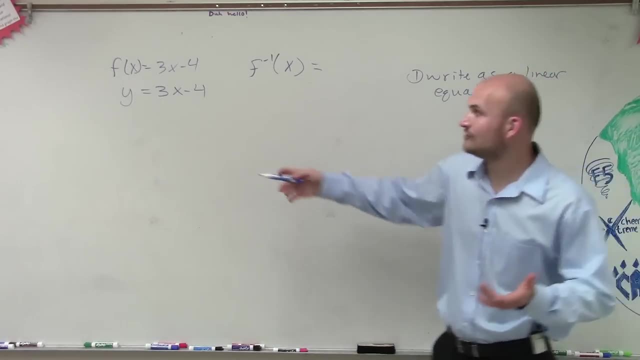 to use x and y's All right. so the first step is just to write it as a linear equation, Because we don't want to do mathematical operations with f of x, even though f of x and y are both your output values if you were to graph it. But we want to deal with y Because step number 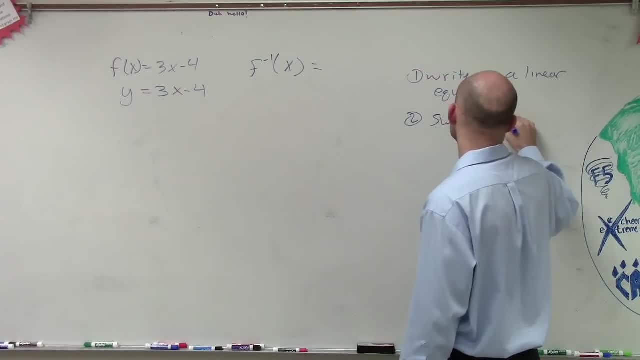 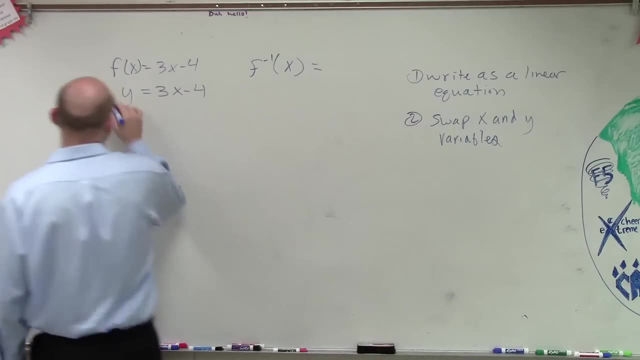 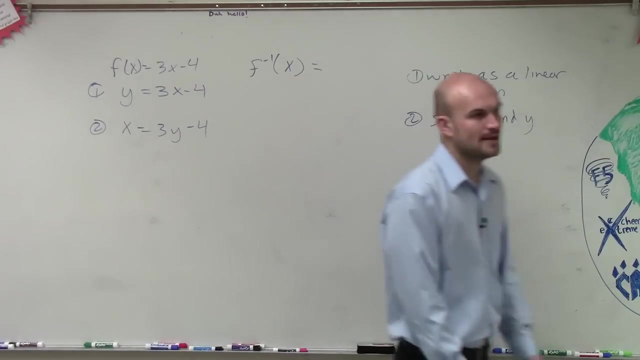 two says to swap your x and y variables. So now we'll swap x and y. So this was step one. Step two: you just swap x and y. Step three: solve for y. So now what we do: solve for y. So you add four to both sides And 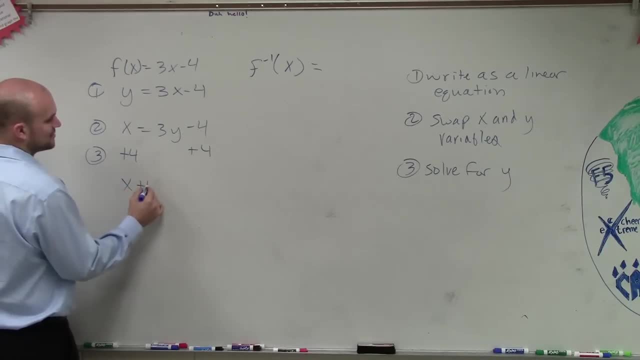 remember, this is a literal equation, So you're not going to be able to get a value. So it'd be: x plus 4 equals 3y, Then divide by 3.. So therefore not yet. So therefore we have x plus 4. 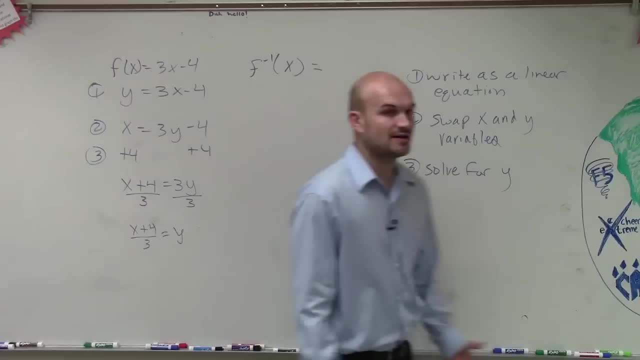 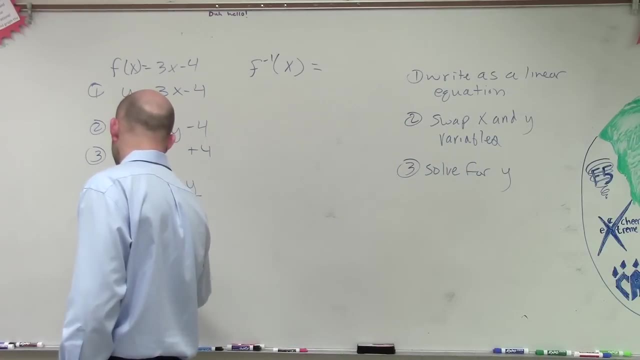 divided by 3 equals y. So I've done now step number three. Can't you simplify that though? We can rewrite this? We can write the y first and write it as 1 third x plus 4 thirds If. 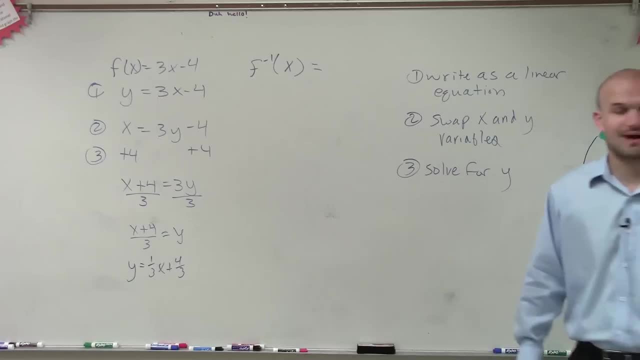 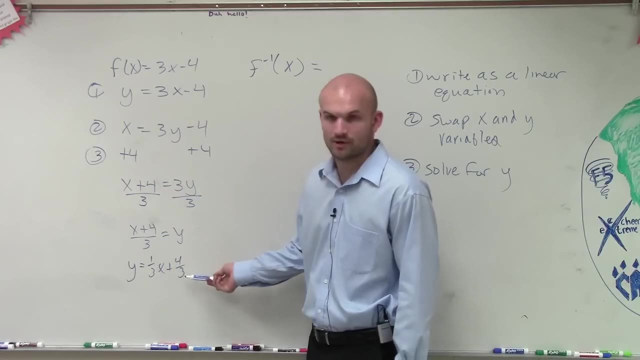 we were going to graph it, if you guys remember graphing it, remember I asked you to graph the inverse. This might be a little difficult to graph, So one thing we can do is divide the 3 into both of those terms. So then we have a slope and a y-intercept, But for this 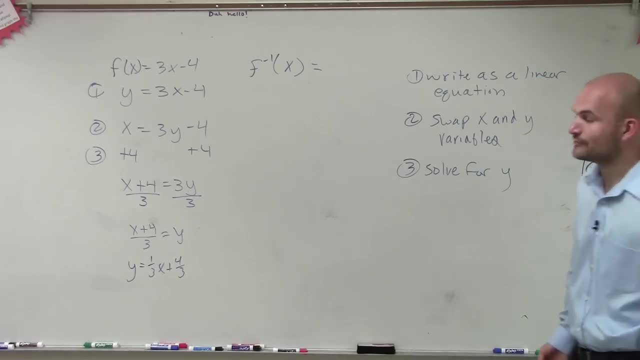 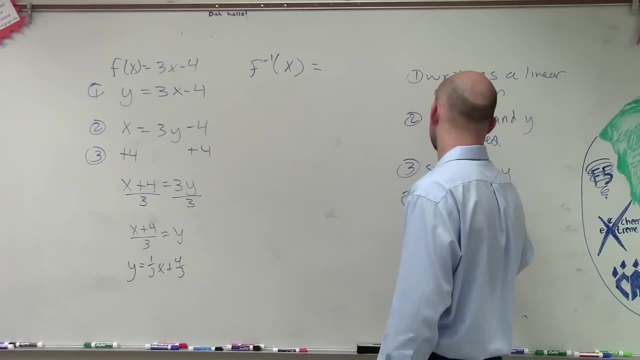 case, I'm not asking you to graph it, So leaving it in that form is fine, But if you were to graph it, you might want to remember how to do that. And then the last step 4, write in inverse notation. So inverse notation, ladies, and. 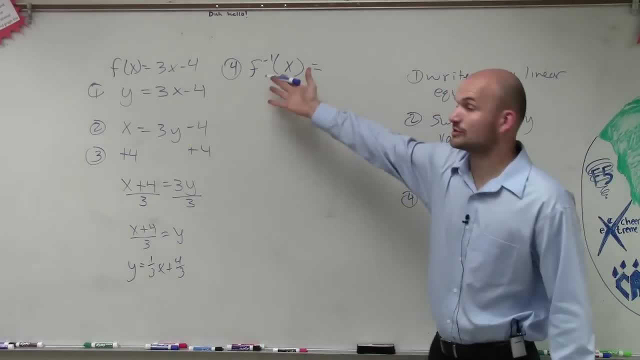 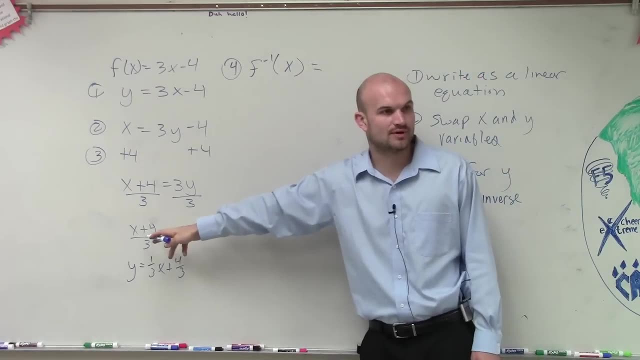 gentlemen. So originally, if I had a function f of x equals 3x minus 4, inverse notation looks like this: f inverse, with that little negative 1 of x equals. what did we say? What did y equal x plus 4..